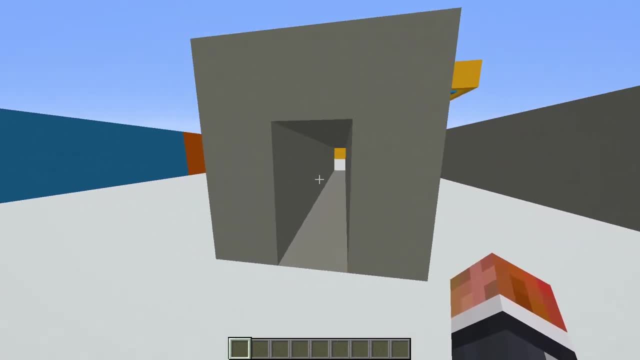 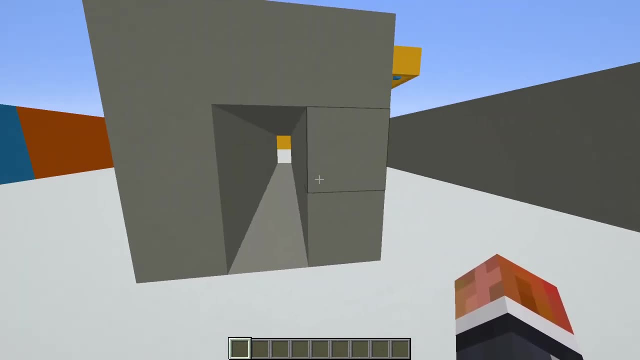 through it in about two seconds, which is pretty cool. And the same thing goes with this tunnel: It takes you five million years to get through, but it's actually really short, which is very interesting. So now we have a little hallway set up and there's a corridor, a big, long corridor. 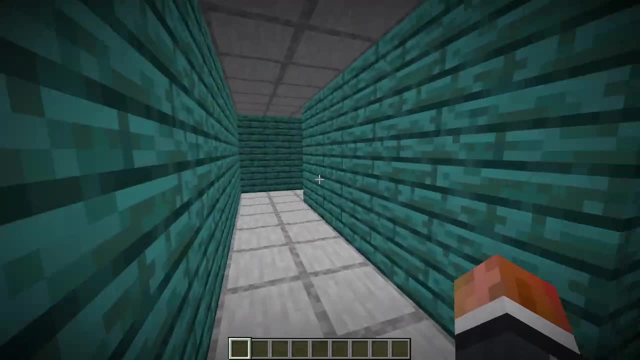 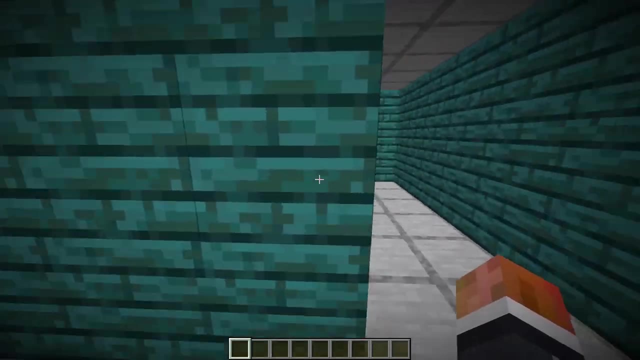 going that way, a little corridor going that way and watch what happens when we just walk down. So there's a big, long corridor over there. we walk down here, we turn another corner, and That's strange. We'll go again just to be sure. Oh, that's also very strange. This shouldn't be. 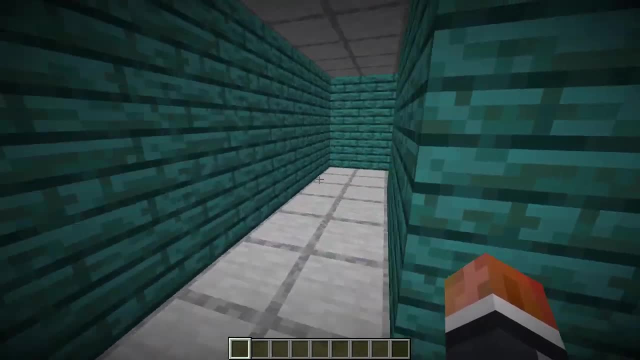 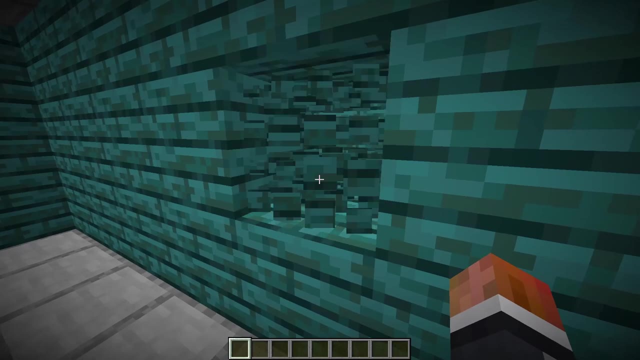 possible? How? Hmm? So yeah, this is a really, really cool non-Euclidean corridor that you can make with this mod. I'll leave a link to the mod in the description. You can do some really cool things with this, so I'll show you some some other things that have been. 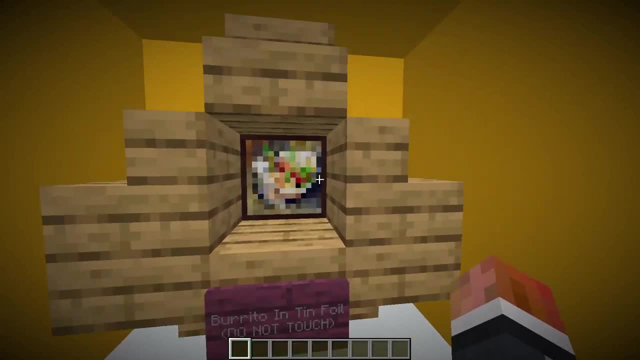 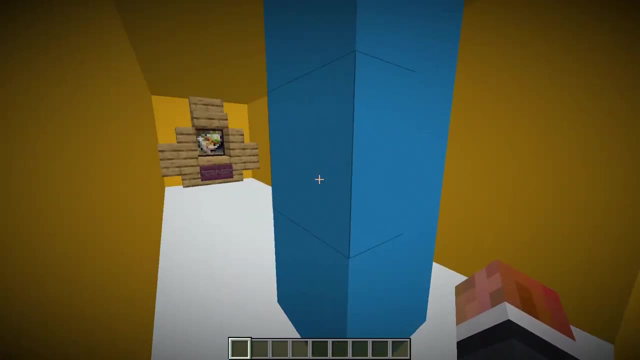 messing around with. So if you take a look in this room, as you can see, there's the classical art piece burrito and tin foil, and it's a very admirable picture. and if we go around this little little pillow that I've set up, Oh what's this? It's gone. and now there's a cake. It's very tasty. 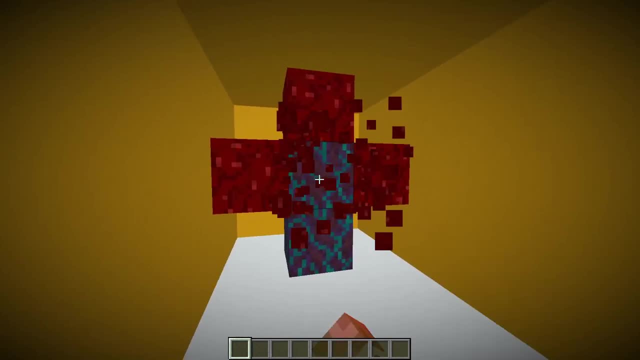 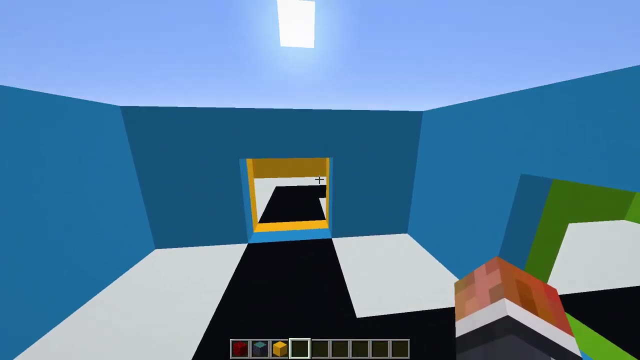 Yes, And if we go around it again then we have this weird nether looking tree. I don't know what to put here. If we take these four rooms with a black square running through the middle and we drop into it and we walk around, suddenly it's not a black square and 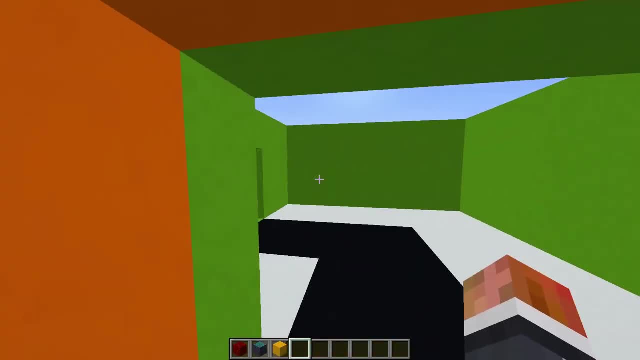 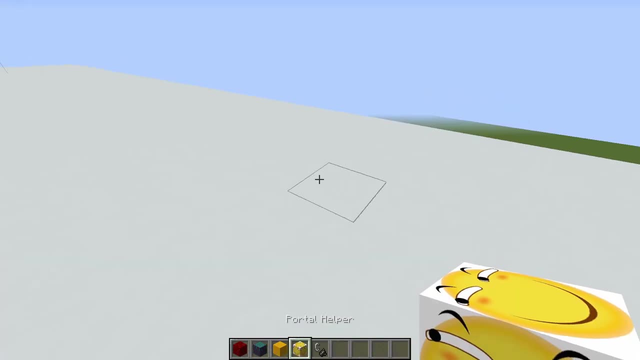 it's a weird squiggly line and I don't know about you, but I think that's pretty weird. So the way that it works is- you've probably guessed by now- there's portals in each of these corridors. So the way that it works is you make a portal out of these. 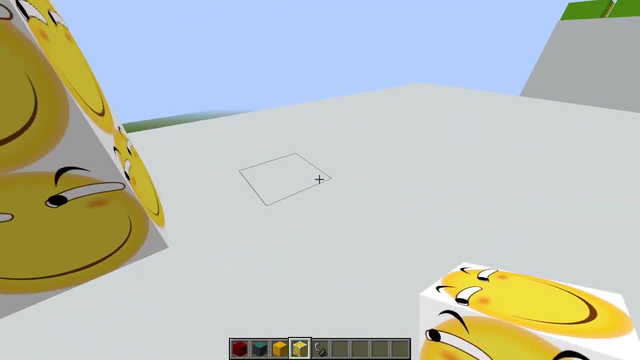 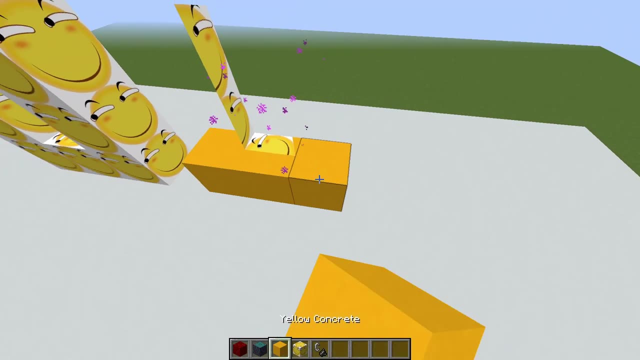 portal helper blocks. Don't ask me why they've got these text checkers, I don't know. So you make two portals, you elide them, stick some blocks around this and voila- Seamless portal. Look at that. Look at how cool that looks. 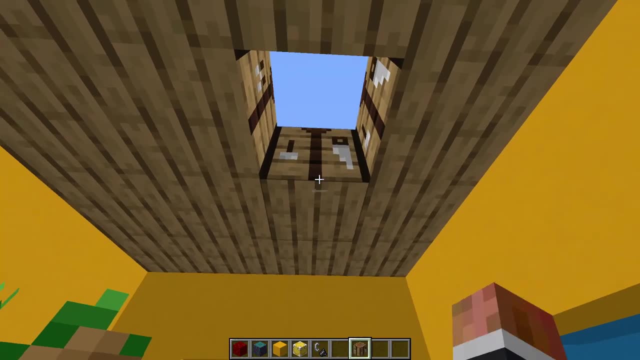 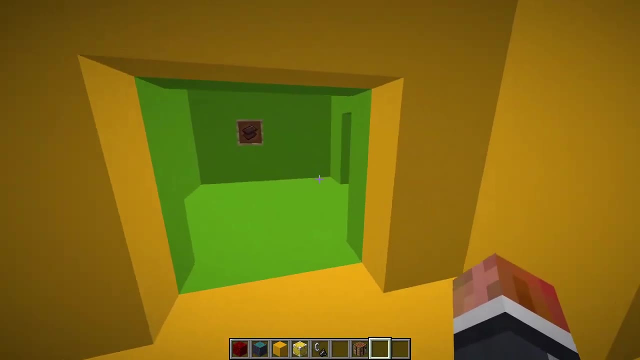 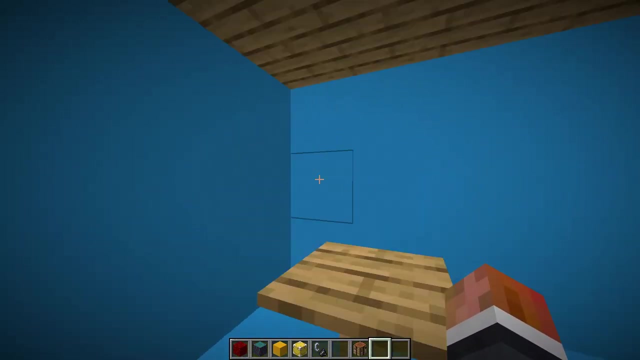 So we're going to this little contraption that I've made. We've got a yellow room with a sapling in it. It's a pretty, pretty swag looking room, if I do say so myself. We've got a nice little green room with some of that in it and we've got a little table in a blue room and I think 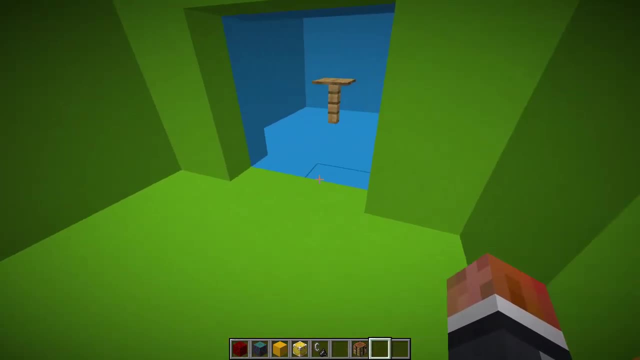 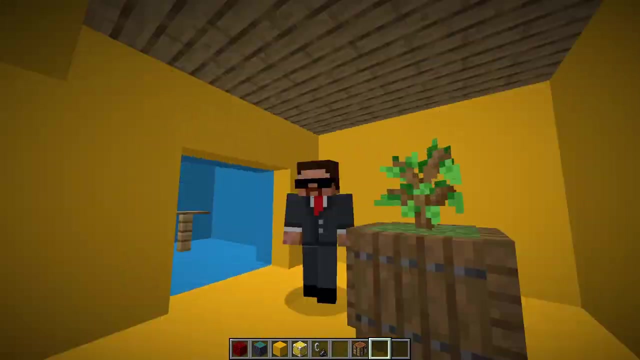 it's pretty cool. So if we start off in here and we take a little walk around, we go yellow, green, blue and- oh wait a second, We're at the yellow room again. I don't know about you, but that that seems pretty weird to me, And so the way that this works is we've actually only got 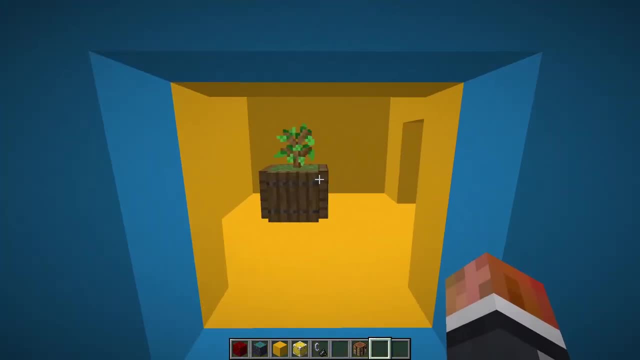 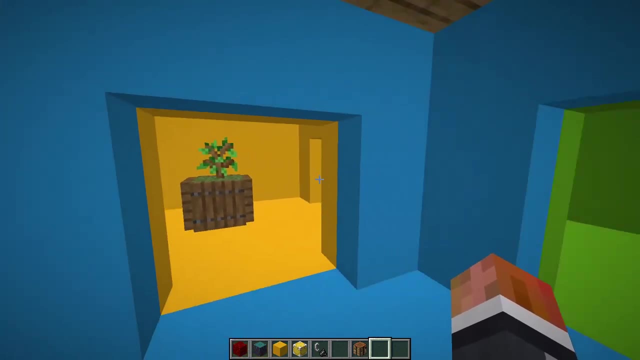 three rooms and we're taking 90 degree turns and we still end up in the first room. What we've done is we've filled four rooms with the space with three rooms, and I think that's actually pretty, pretty epic, if I do say so myself. You could actually do this the other way around as well. 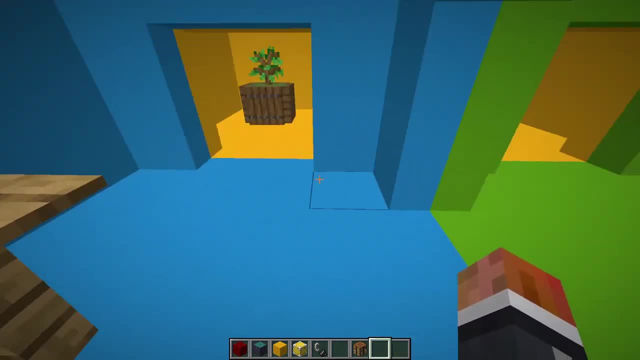 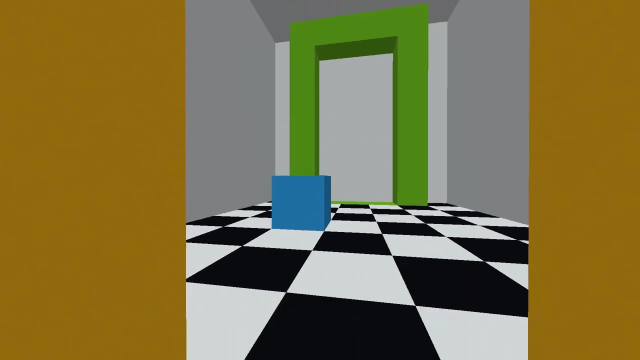 You could have the space of four rooms and you could stick as many rooms as you wanted in there. And another thing that I think is pretty cool is if we're in this big room here and if we actually fall into the smaller version of the room, and you could keep this going, you could repeat this. 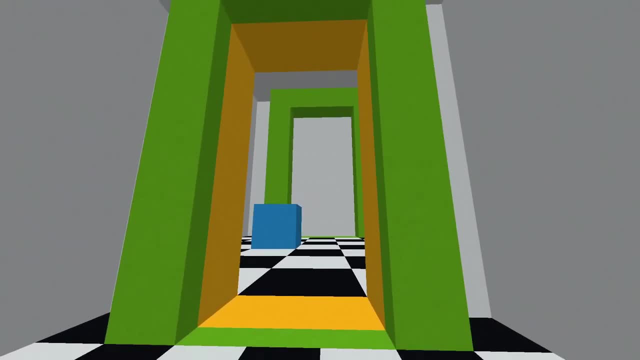 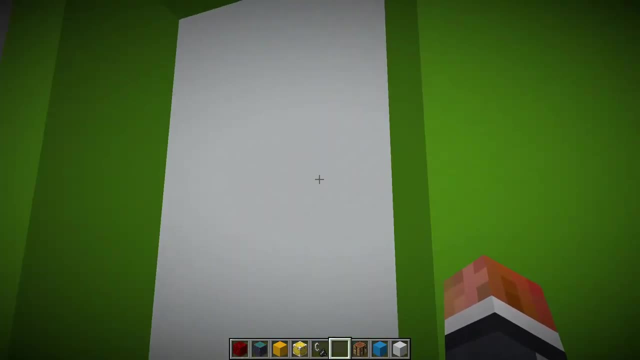 I can't be arsed building you know six rooms worth getting exponentially bigger- of blocks. I could not do that. I didn't have the patience. But if you really wanted to, you could. you could keep this going for a while and seem like you're getting smaller and smaller. 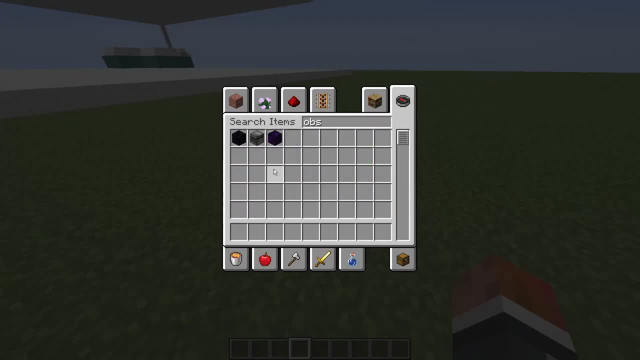 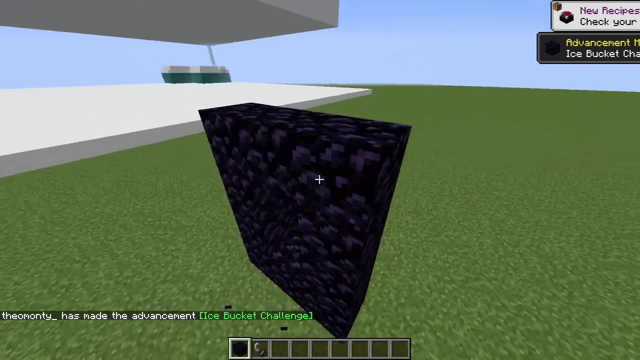 The mods actually does some cool stuff as well. You get- you just get a nether portal. It actually loads in the nether- You've probably seen this before in some other mods- but it pre-loads the nether and sticks. It sticks to the nether in it so you can- you can see into it through the overworld. 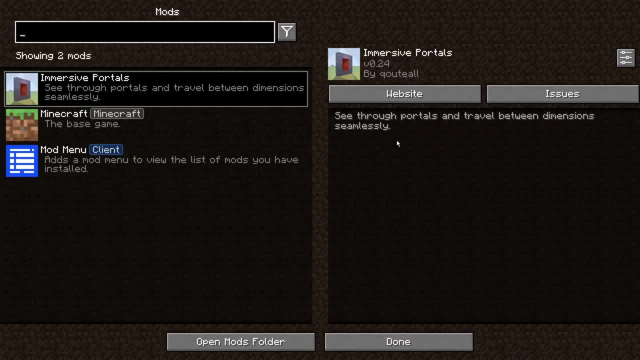 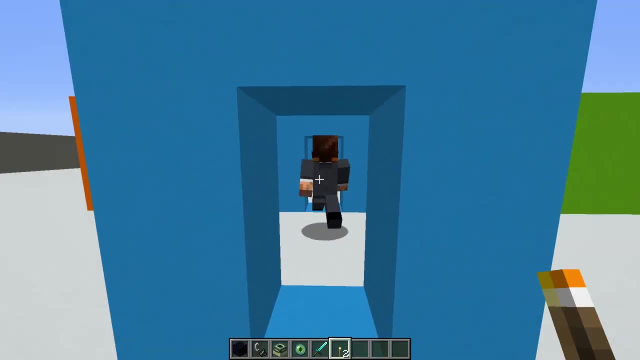 I think that's pretty cool. So yeah, that's the extent of this mod. If we go into options, we'll just stick around yourself and portal Set that to true so we can see our beautiful backs. So yeah, that's pretty much the end of the video. If you did like it, please do subscribe, because 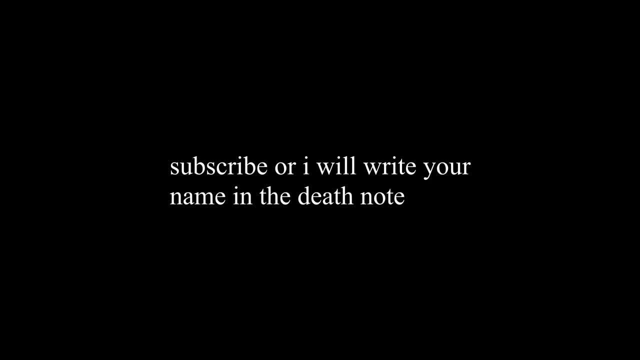 because I want subscribers And I'll see you guys in the next one.